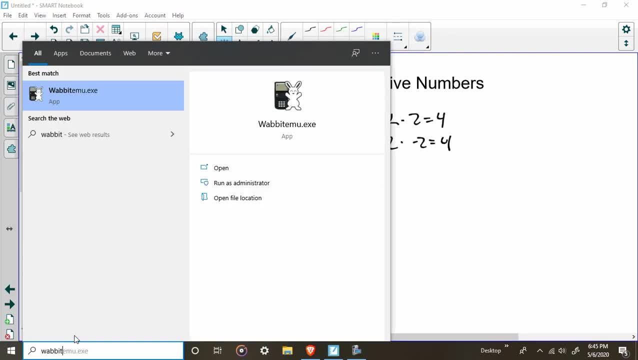 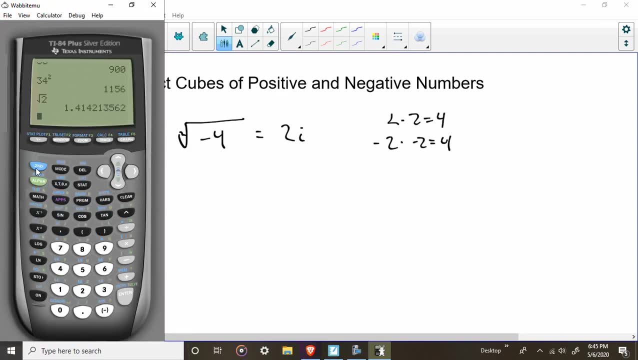 If you plug that into your calculator- and I'll plug it into my calculator now that it told you no, That it told you no, There is no answer to that problem as far as your calculator. So that's the point. So if I said, hey, what's the square root of negative 4?? 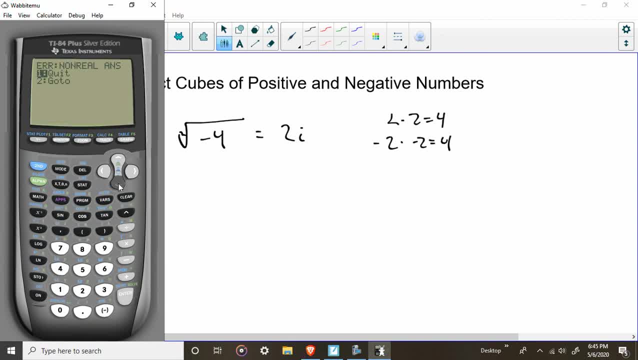 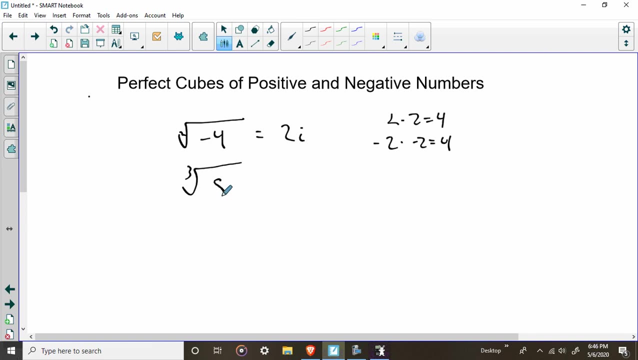 Your calculator would say: I can't do that And it says non-real answer. In other words, there's an imaginary answer, It's not a real answer. okay, Okay, But we said, when you have an odd index like 3, if I said, hey, what's the cube root of 8?? 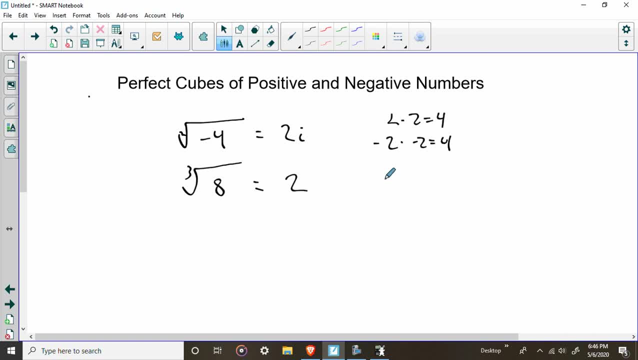 Well, we know, the cube root of 8 is also 2.. Well, because 2 times 2 times 2. Makes 8.. We said the little 3 there means what number times itself 3 times makes 8, right. 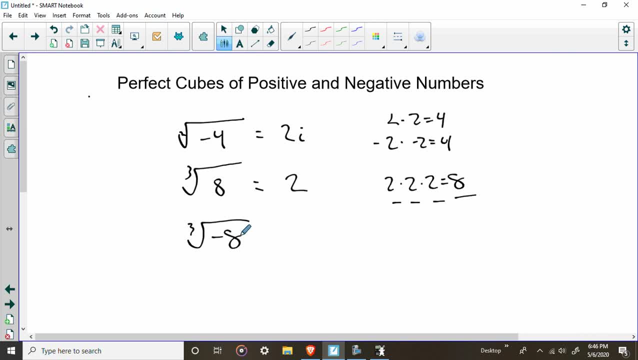 But we also said, though, if I had a negative number, I can now take the cube root of that. I can say: hey, what number times itself makes 8?. And all we had to remember was that it's the same number here. 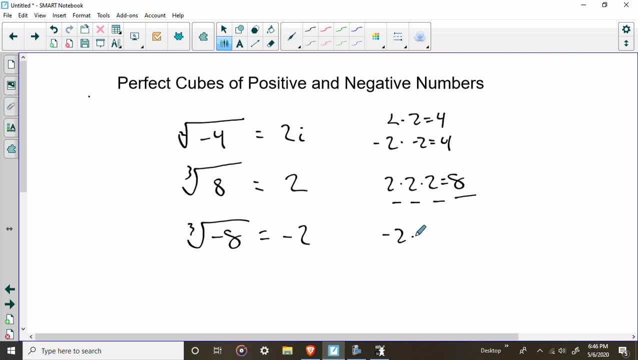 It's just negative because we can multiply this, right here We were talking about odds of even numbers, right That? because I'm multiplying it by itself, an odd number of times, a negative times, a negative is a positive times, a negative will be a negative answer, right? 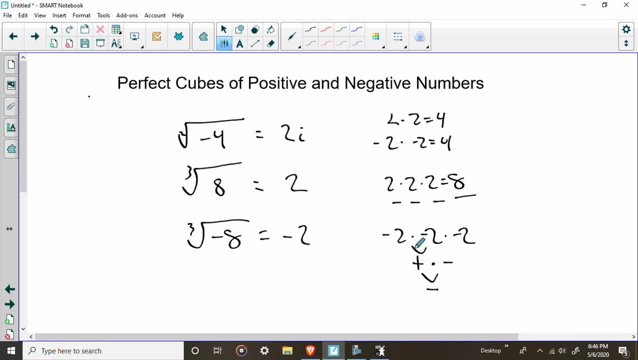 When we start multiplying these things, then we will get a negative. We have an even number. then we would always get a positive right. Even number: 2 times 2 is 4.. Negative: 2 times negative: 2 is 4, right. 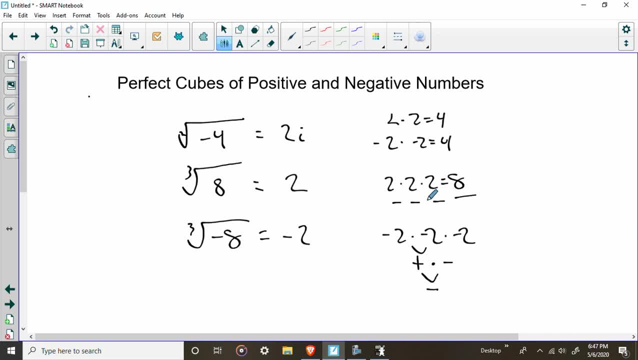 We have an even number of things we're multiplying here, since we have 1,, 2,, 3.. An odd number of things we're multiplying, we can get a negative. okay, So your task for today is really just to get a negative. 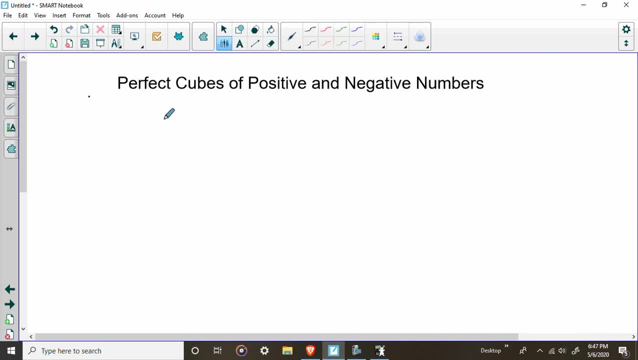 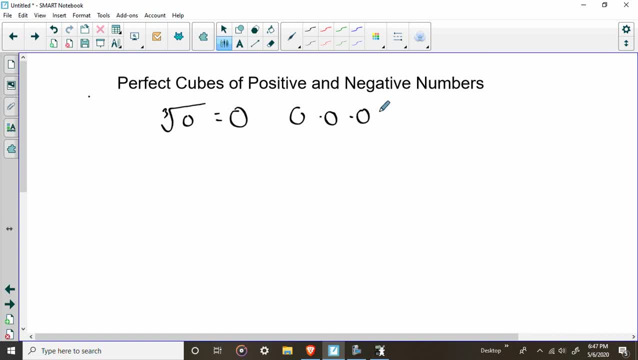 Well, it's 0.. Why? Because 0 times 0 times 0 equals 0.. If I said, hey, what's the cube root of 1?? It is 1, because 1 times 1 times 1 equals 1.. 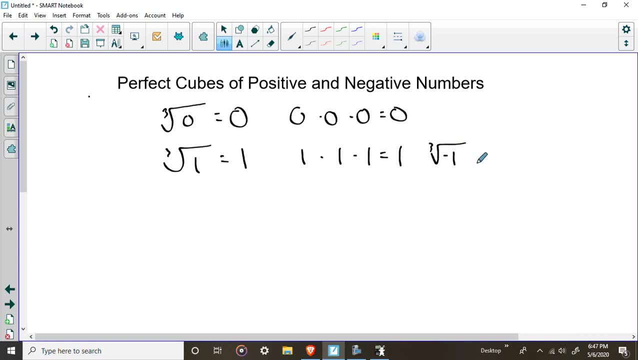 If I said what's the cube root of negative 1, you would tell me that is negative 1, because negative 1 times negative 1 times negative 1.. times negative 1 equals negative 1,. okay, Your other common cube roots, the cube root of 8, is 2.. 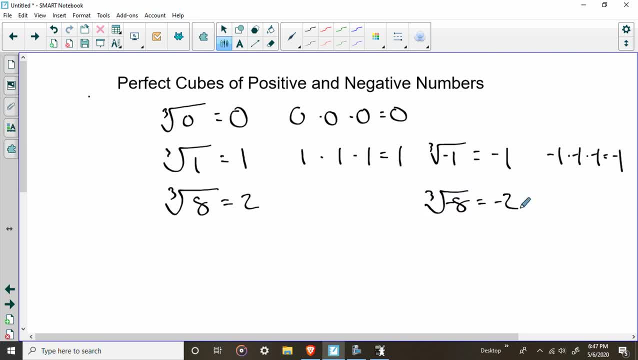 The cube root of negative 8 is negative 2.. The cube root of 27, and then your next ones are the cube root of 64, and your cube root of 125,. okay, So these numbers, if you haven't noticed, are going to get real big, real fast. 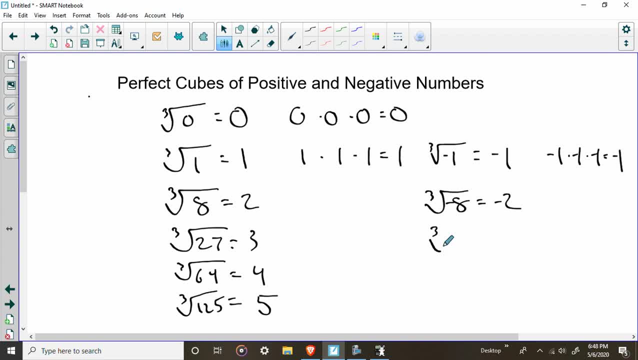 Okay. So for the most part, a lot of this is just going to be plugging it into a calculator. So if I said negative 27,, it would be negative 3.. If I said the cube root of negative 64,, it would be negative 4.. 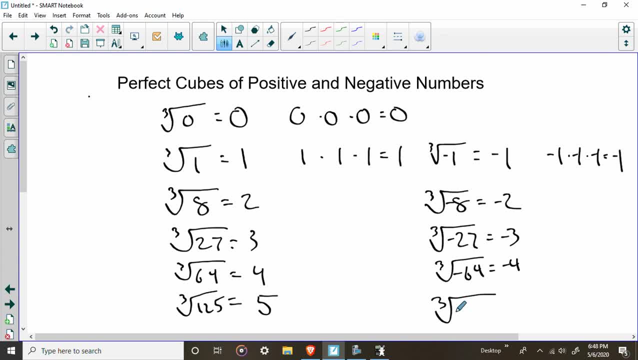 And that's the big thing we want to take away from this- is that you're allowed to take negative cube roots. 125 is going to equal negative 5, okay, So I'm going to show you guys how to do it on a couple of different calculators. 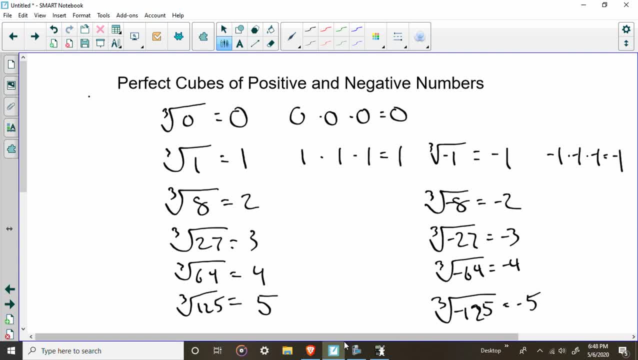 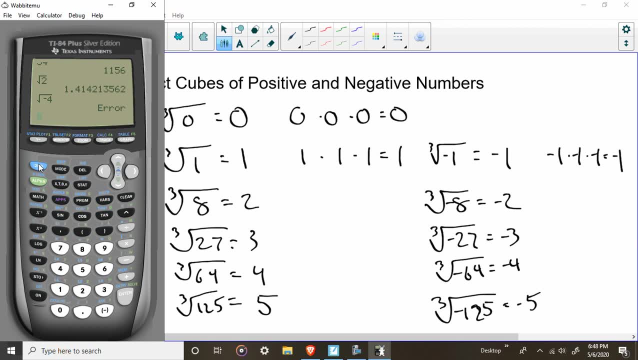 You can choose the method that works best for you. If you're using a TI-80 for any Texas instrument, even if it's a basic TI-34, you're going to press- I believe it's math. You're going to go down to number 4 to get the cube root. 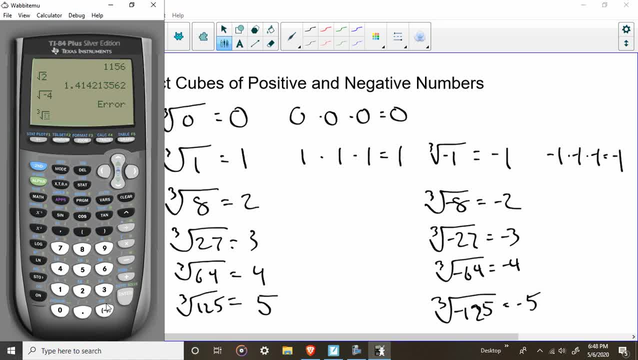 And now you're going to be able to put in negative numbers. If I say, hey, what's the cube root of negative 125?, You can say it is negative 5, and it will give you an answer. So again, that's math. 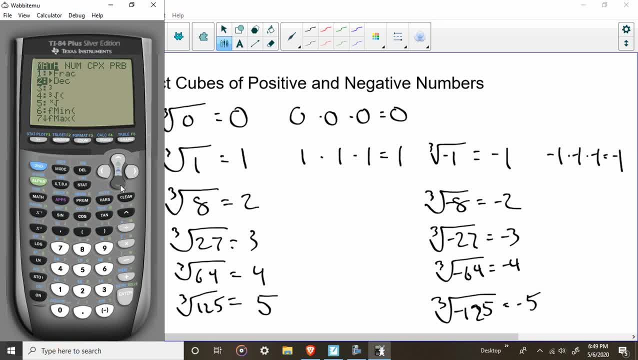 And I'm going to go down here to Number 4.. You can either click down here and press Enter or you can press the number 4.. And if I say, what's the cube root of negative 10,000? Negative. 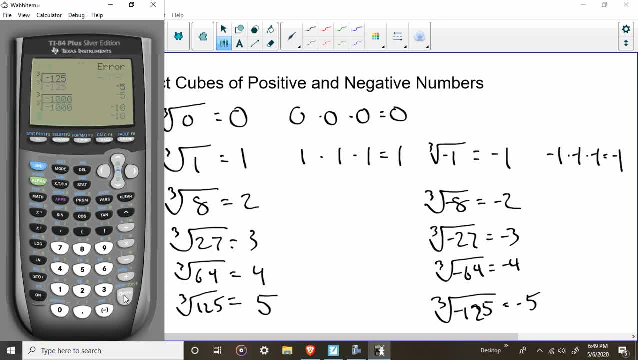 I'm sorry, negative 1,000.. It would tell you that's negative 10, right, And it will tell you other numbers. It will tell you: you know things like: what's the cube root of 5?? Well, there is a cube root. 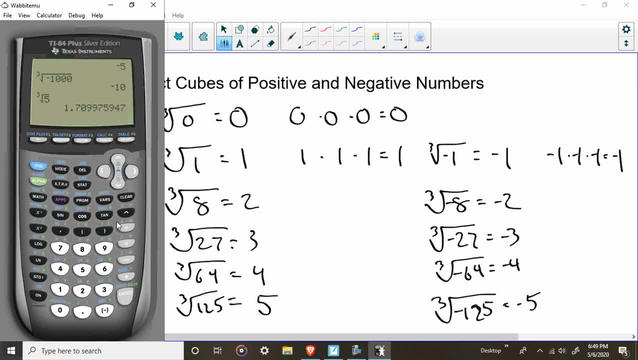 This number times itself, whatever it is, will give you 5.. So if I raise that, If I raise that number to the third power, it will give you 5.. So, just like square roots, a lot of these are going to be irrational numbers, okay. 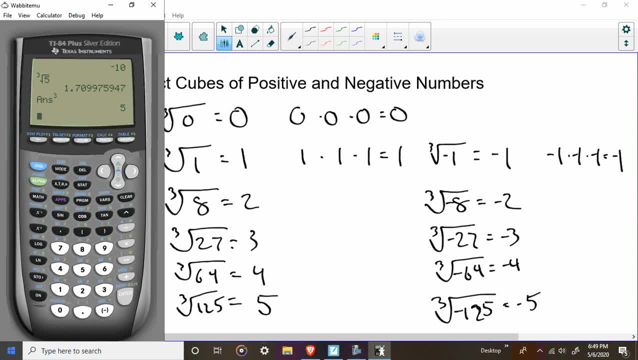 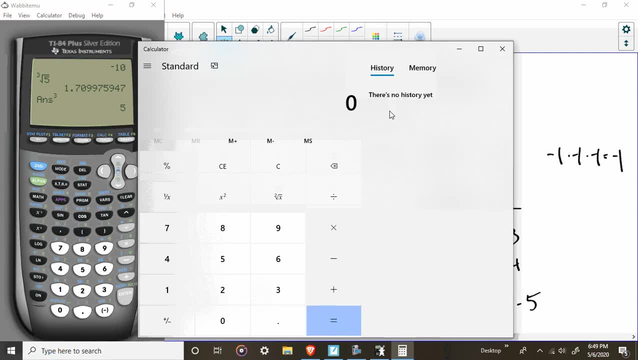 But the point is, you put it in your calculator If you are using. Oh I don't know If I bring up just the regular Windows calculator. I don't have an. I can't bring an iPhone. I know a lot of you guys are using iPhone calculators. 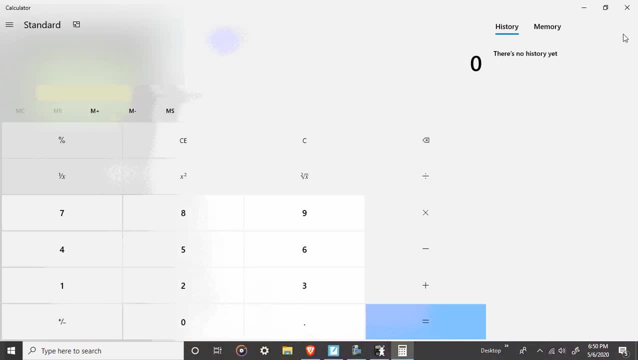 If you turn your iPhone calculator sideways, How do I get this into a standard scientific Um? A lot of times, A lot of times on regular calculators, if you notice where is my cube root. But do I not have? Are you serious? 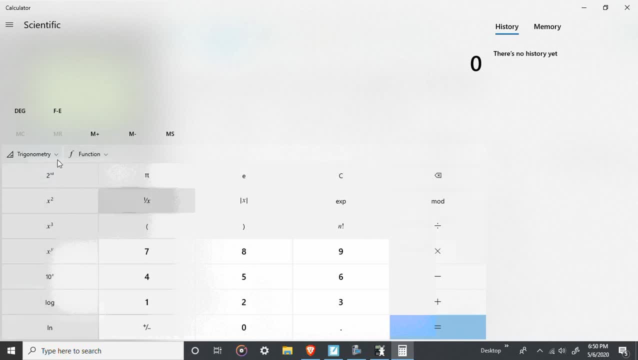 Do I not have a cube root? I got squares. I got square roots. I got All right- Third time Currency volume length areas. But I got all these calculators. I can do Programmer, Oh God. 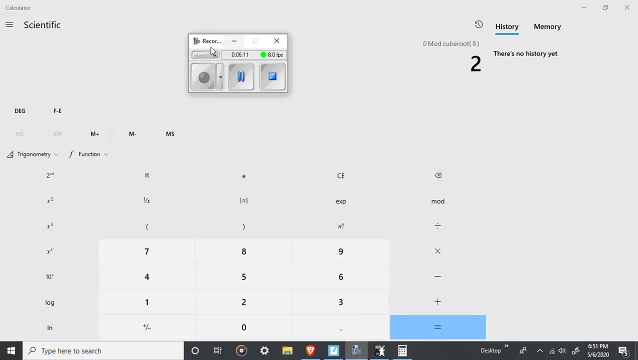 Hold on Timeout. Okay, I found it. Sorry about that Again, on your iPhone calculator. one of the things you're going to have to do: How do I clear this thing? One of the things you're going to have to do on a lot of cases on an iPhone calculator is you're going to have to put in the number first. 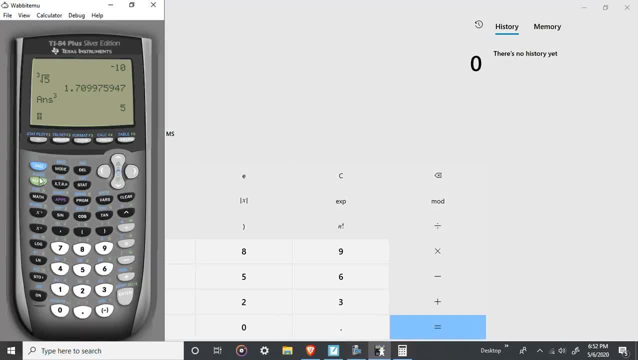 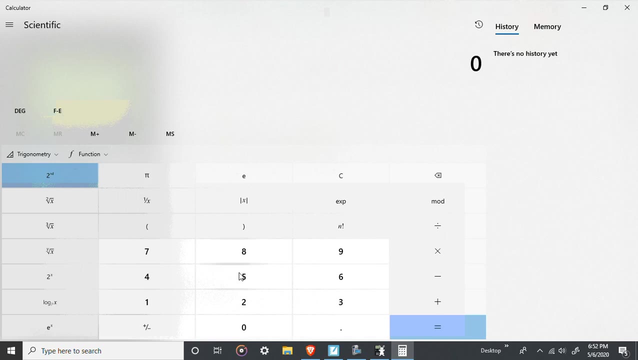 So, whereas on a TI-84, you press the square root or cube root or whatever root you want to take, you're going to put the cube root and then put the number, Okay. But when you want to do it on a lot of scientific calculators, or your iPhone calculator is you're going to put in the number first, then you're going to press the cube root button. 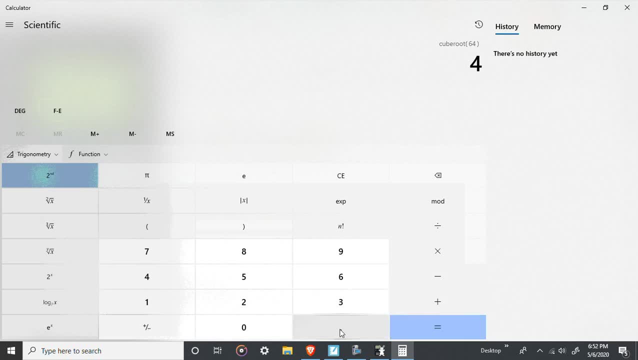 Okay, So it'll be there. So if I said, hey, what's negative, If I said, hey, what's the cube root of negative? four, Again, what am I going to have to do on a lot of calculators is you're going to have to put in? 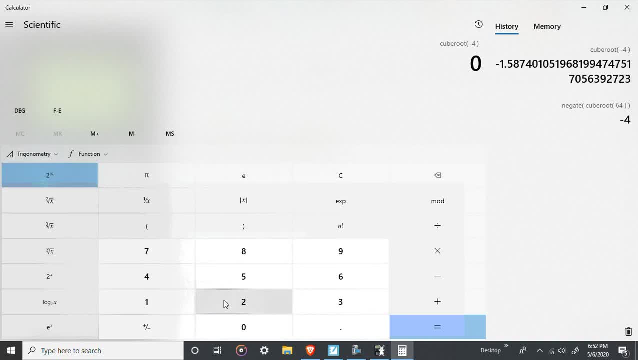 Let's put in the number first. We'll say 27, then make it negative, then take the cube root of it. Okay, So you might have to, You might have to work with it a little bit backwards, but you should be able to. 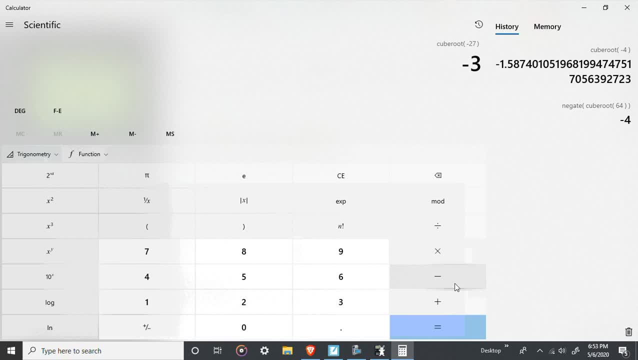 I'm sorry I can't bring up an iPhone calculator on the screen. I looked online real quick. I know I paused it, You guys didn't know, but a couple of minutes passed I couldn't find one online. But again, it should be the same kind of protocol on an iPhone calculator. 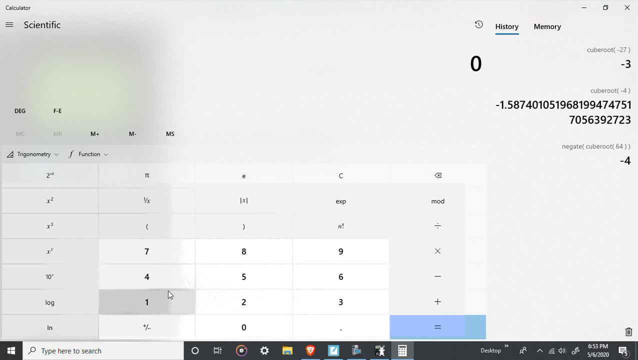 So again, let's say I want to take the square root of negative 125.. I got to put in 125 first, then I have to make it negative, then I have to take the cube root. Okay, So give that a try. 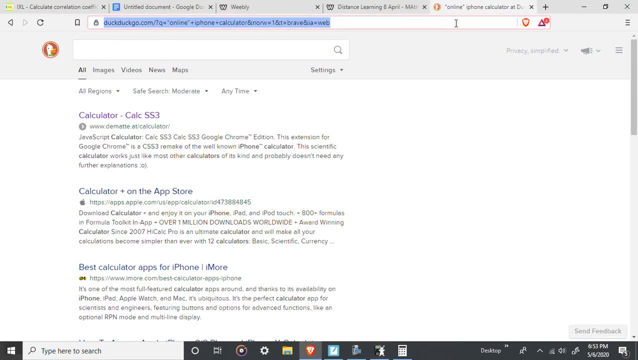 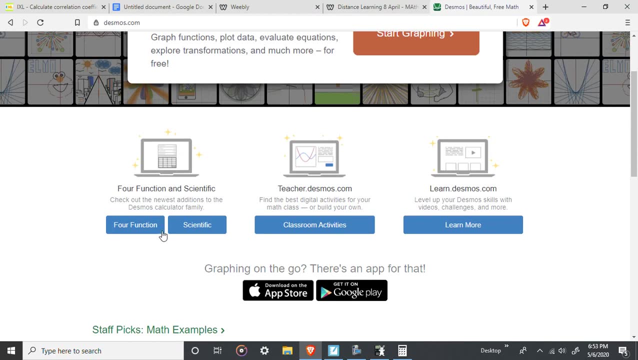 Okay, If not, you guys get stuck with that Again. you can always use Desmos. Desmos has a free scientific calculator you can use. It's pretty user-friendly and you can bring it up on a touchscreen. so that's really nice. 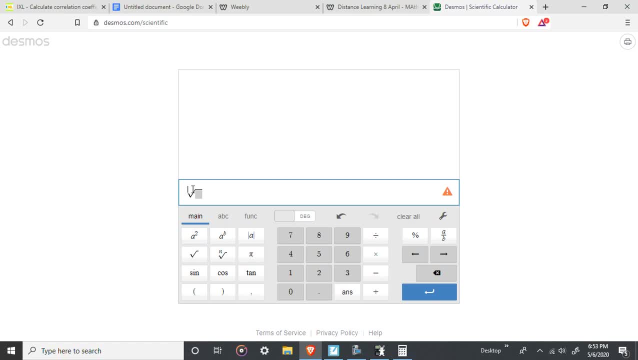 All you have to do is you have to press the nth root, put a 3 in there and then plug in whatever number you want. So negative 125. Okay. And what you can do is you can actually just leave it like that and you can just kind of change the number that's in there. 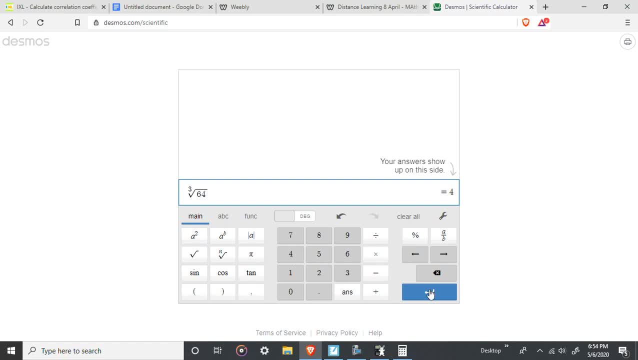 and it will give you kind of your answers as you go. Okay, So again. big thing I want you guys to take away today is: it's okay to take the cube root of a negative number because we said it has an odd index. 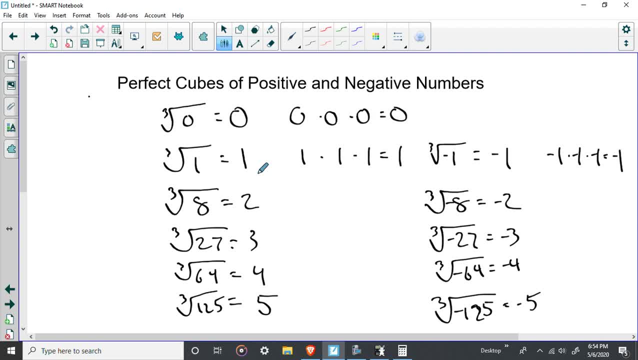 Okay, And all you're really going to have to do is, if it's any number that's really larger than this, you're just pretty much going to plug it into a calculator. Okay, The numbers get so big that they're really hard to comprehend. 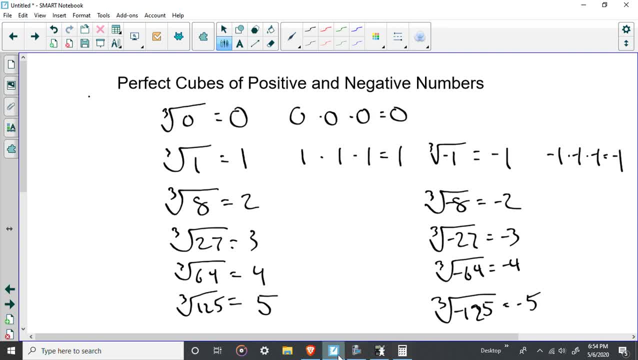 So anyway, I hope you guys have good luck with that. Try the iExcel skill. I recommend it and I will talk to you guys soon. Thanks, Bye.